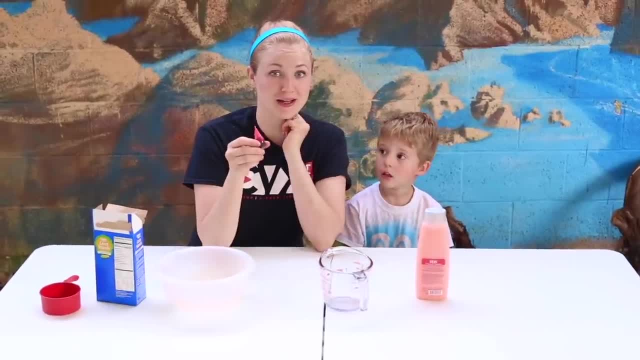 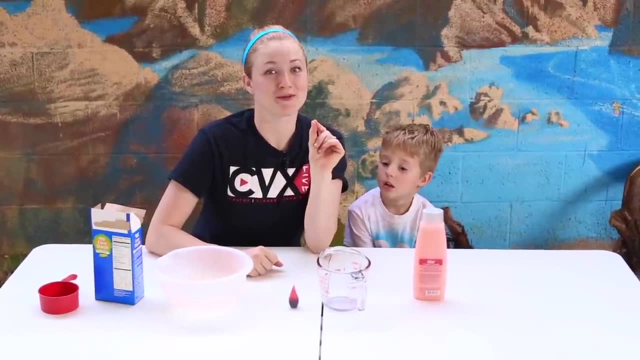 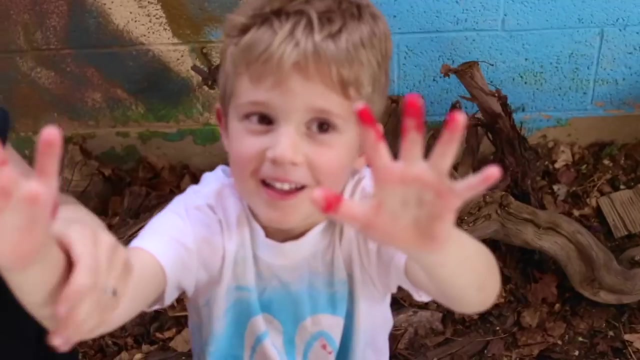 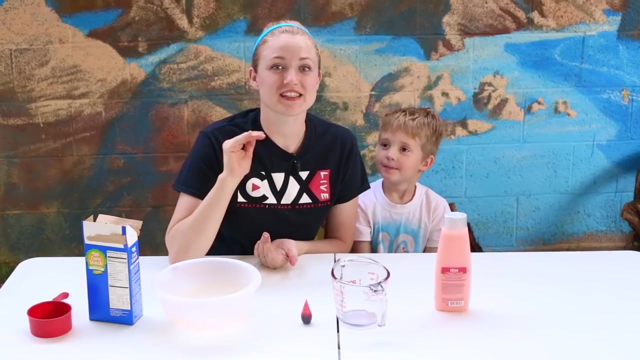 I noticed that somebody had gotten into the red food coloring, and I just figured out who, because I literally caught them red-handed. Check that out. You were caught red-handed. You got into it, didn't you? Are you naughty? So this is the most smooth play-doh recipe and simple, that you could possibly get. 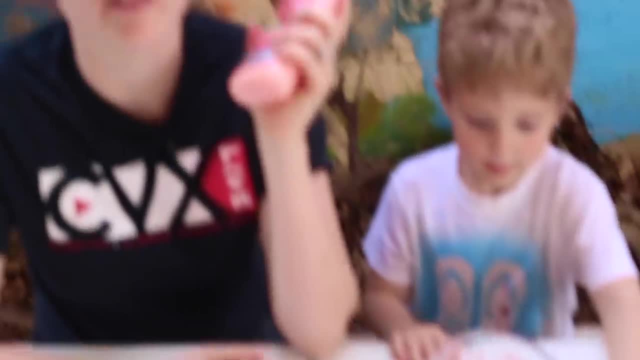 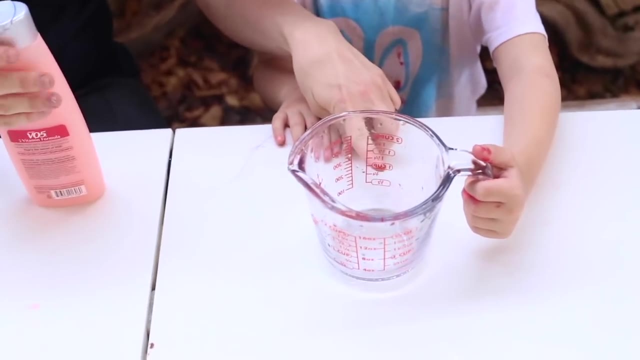 So this is what it takes: One cup of a very cheap, the most inexpensive conditioner you could possibly find. Corbin, can you do that? Can you put it all the way up to the one right here? Yeah, All the way up to the one. 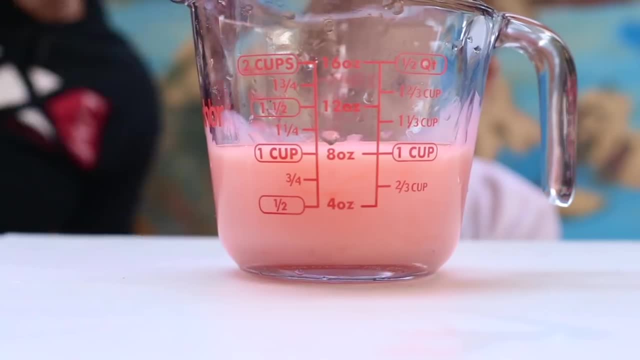 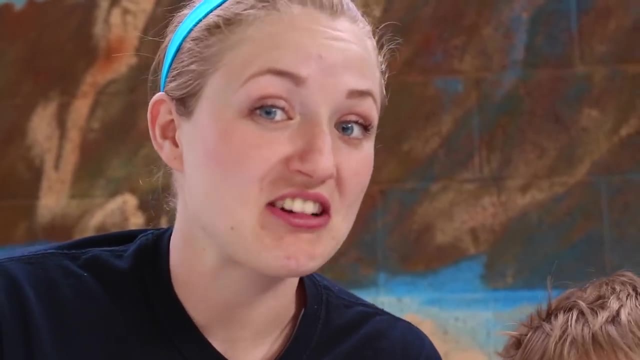 Is that enough? Smooth it out for a second. Yeah, one cup, There we go, And the trick with this is making sure that it's a conditioner that you like the smell of, because you're gonna be smelling it a lot, I'm gonna put in a couple of drops of food coloring and then you can stir it, okay. 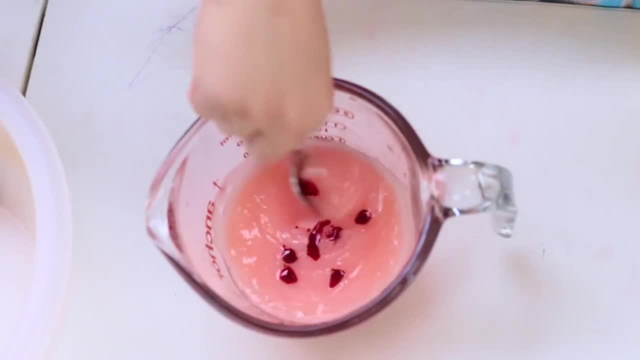 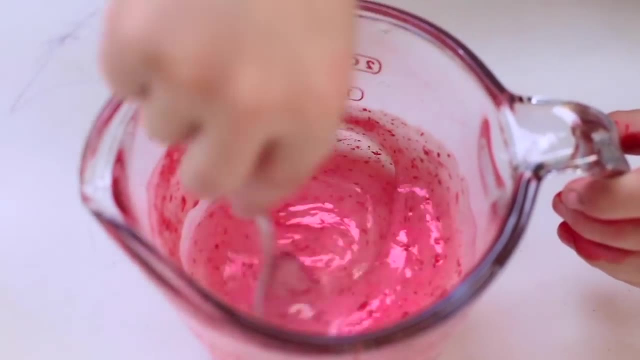 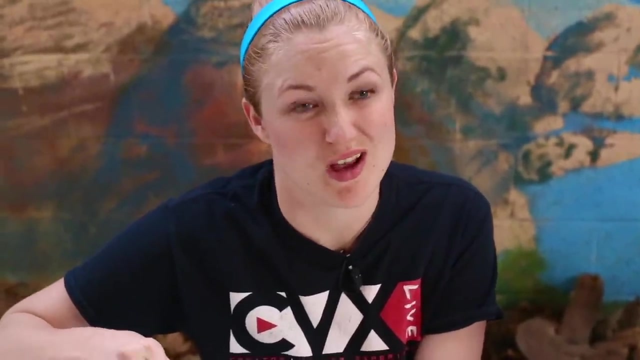 Alright, Okay, go ahead and stir it. Wow, it's not mixing very well. Well, I guess we'll find out if it mixes once we add in the cornstarch. Alright, the cornstarch is super cheap. It's gonna be really easy to mix this together. by the way, 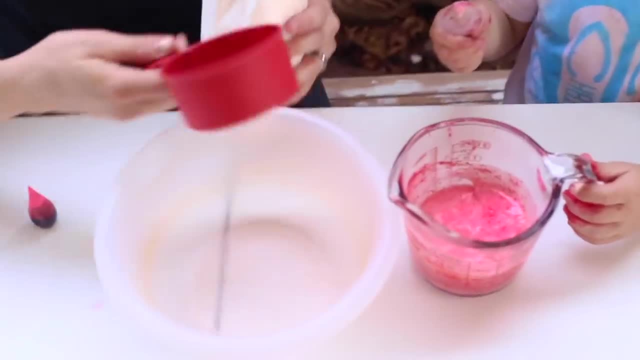 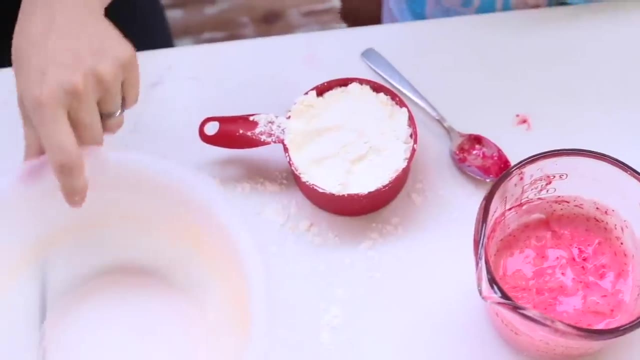 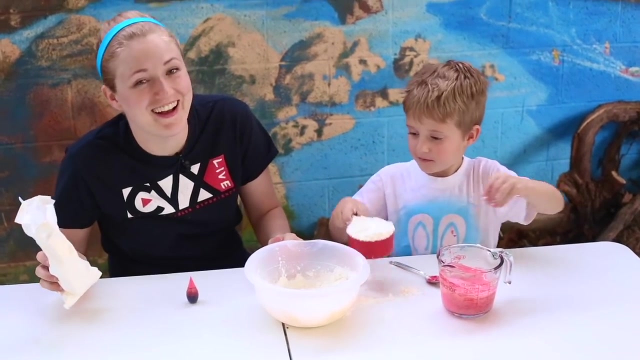 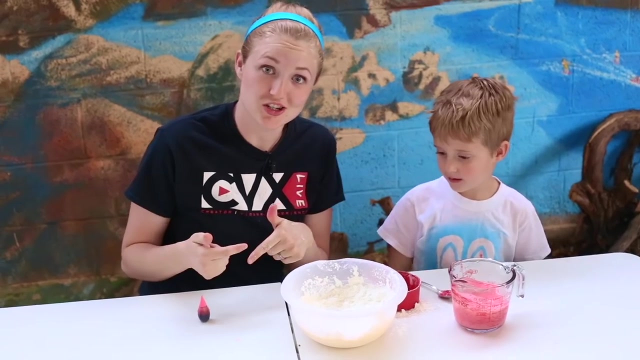 So here's our cornstarch We need to put in this bowl. Are you ready to help me with this Corbin? Two cups of cornstarch- There we go, Put it in here. You are a professional, Good job. Now we're gonna put the conditioner and the cornstarch together. 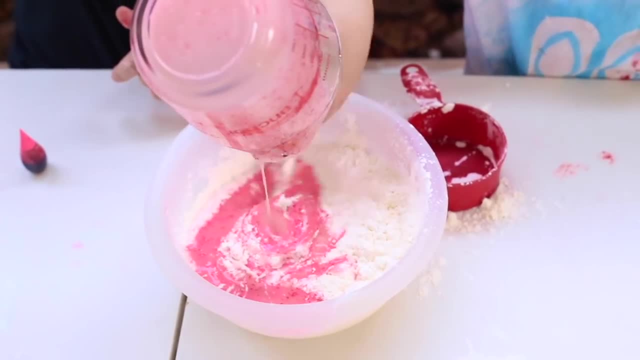 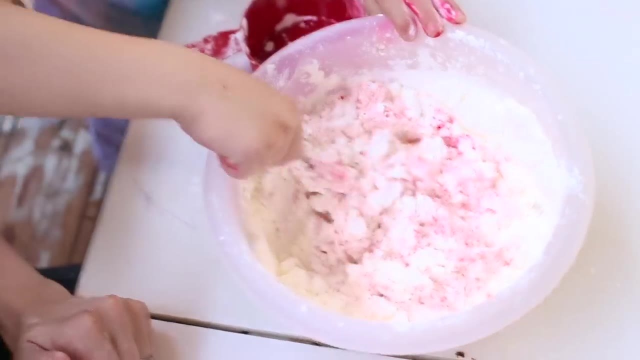 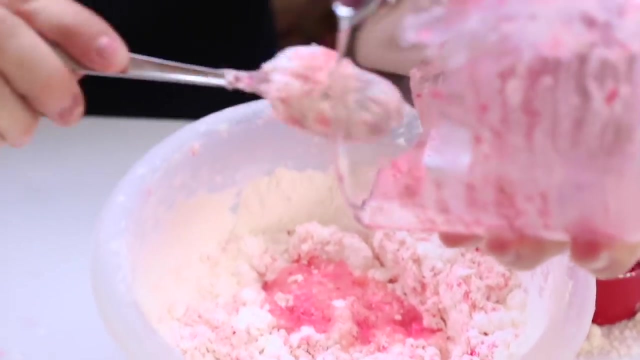 Okay, stir it all together. This is meshy. I think it might be time to get our hands dirty. Let's make sure to get it all out of there. That smells good, doesn't it, Corbin? Yeah, I made sure to get one that smelled like fruity and not like soapy, because I like that better. 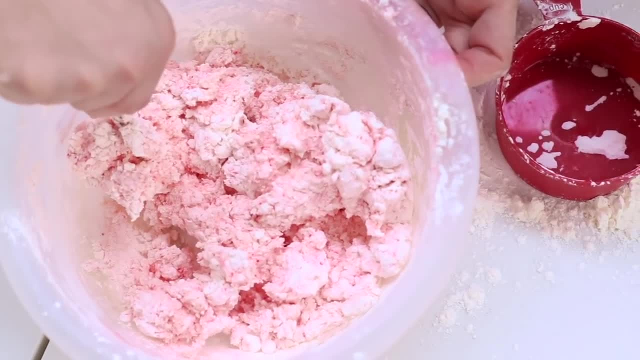 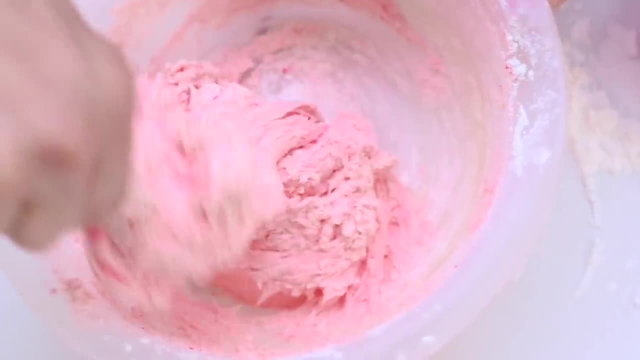 Are you sure you want to help me play with it? Yeah, Are you sure? Yeah, Okay, Oh, my goodness, It looks so pretty. This looks edible. This, you know what this reminds me of? It's cornstarch and conditioner, but it totally looks like pink frosting to me. I could.